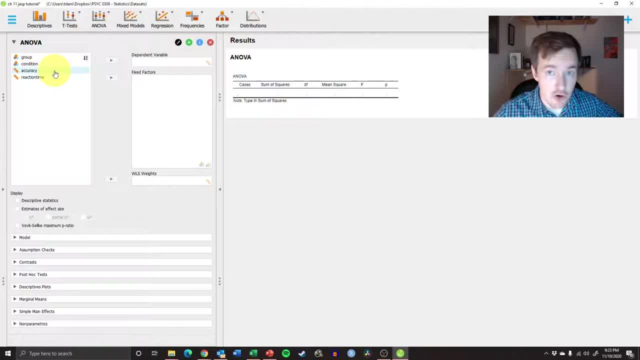 If I were to do both at a time, that would be called a MANOVA, which is multilinear And is beyond what I want to trust right now. So instead I just want to look at these one at a time. So I'm going to go with accuracy first. 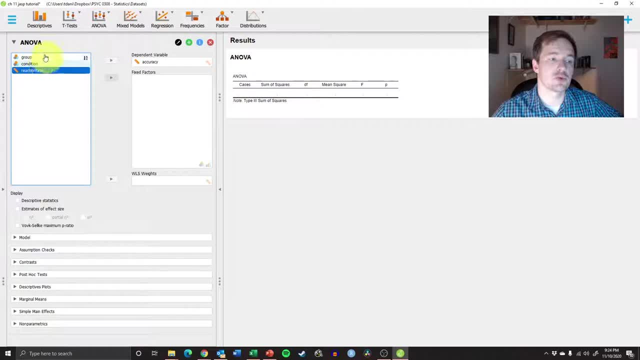 So I'm going to throw accuracy in the dependent variable And now I can pick between these possibilities. I can throw a group in here and then it will analyze accuracy by group, Or I can throw a condition in there and it will analyze accuracy as a factor of or as a product of condition. 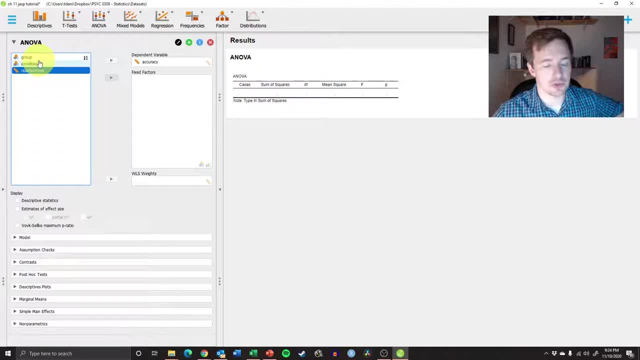 Or I can do both of them, and that is what we'll do. But first I want to just look at it in terms of group. So I just throw in group right here and we can see what appears to be a significant effect. 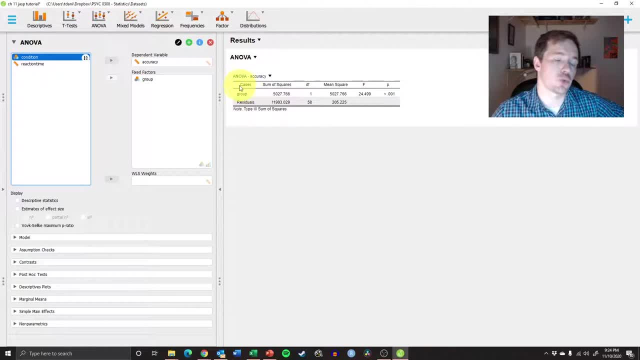 The way that you interpret this is basically group is your between variable sum of squares. Residual is going to be your within subject sum of squares, And so, as we move across, you can think of this as like your between group sum of squares. 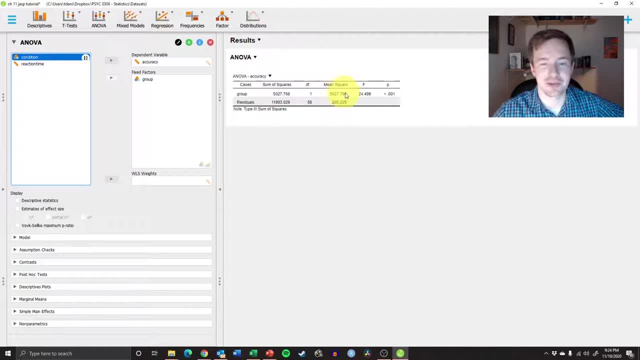 your between group degrees of freedom, your between group mean square, and then, finally, your F value, which, of course, is going to be your F value is dividing your between group's mean square by your within group's mean square. So that's where that value comes from. 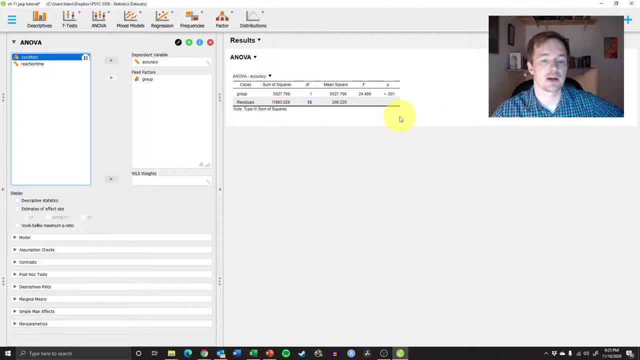 You can see, this is less than 0.05, so we feel successful here. But yeah, so this is not maybe too surprising, because we could have done this with a t-test. And just to show you, I can go over to t-test, I can go over to independent samples. 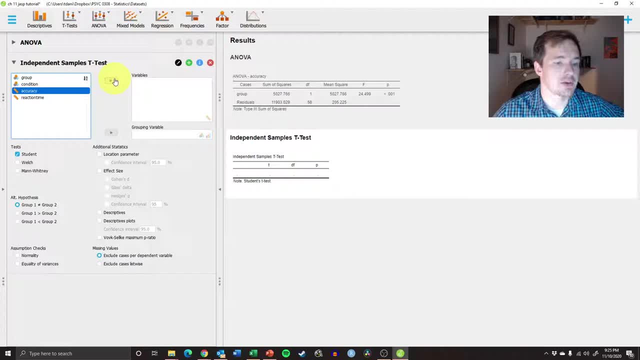 and then I'm going to, I'm going to group the accuracy by group, the factor that I have here, and you're going to see the exact same thing. Of course it is very significant, Okay, but that's not what we want to know. 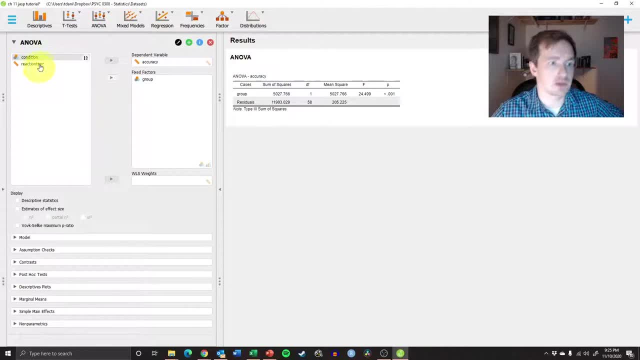 What we ultimately want to know, what we're dying to know, is whether or not group and condition together give us anything interesting, And so what we're looking at here is the between subjects value, and this makes it a two-way ANOVA. 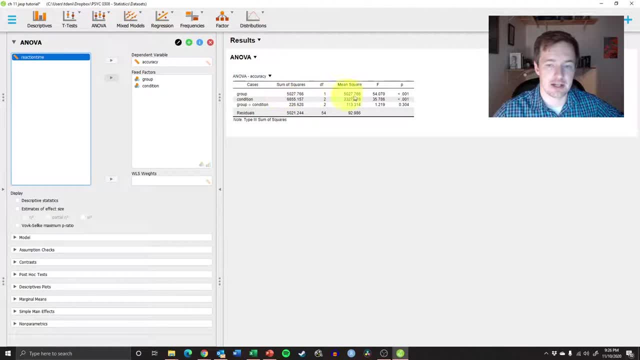 So we have group: Group is a between subjects factor, You can see that it is significant. Condition as a factor, you can see that that is significant. And then group by condition, so this interaction variable, and we see that that is not significant. 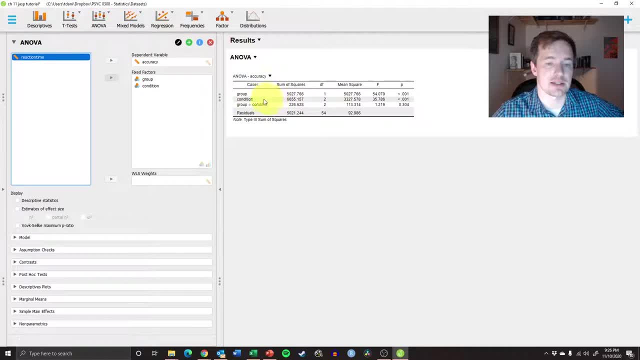 If it was significant, then we would need to do some post-hoc tests to better understand what's going on with that data here. Now, the way that you can do that is going to be at this nice little post-hoc test button. You click on this and it gives you lots of different ways of splicing the data. 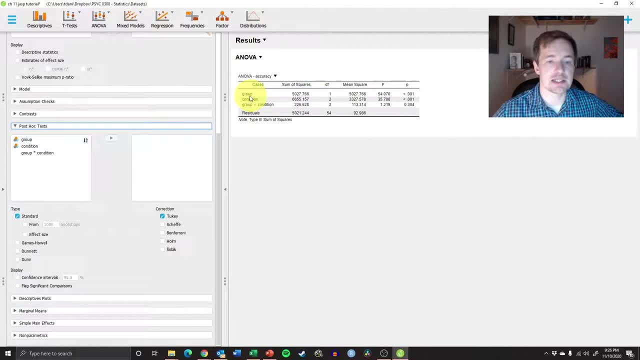 And because I see that group is a significant variable and that condition is a significant variable, I don't know which of those variables matter. Are they all affecting the data, or is it that one of them is different than the other two? We need to find that out. 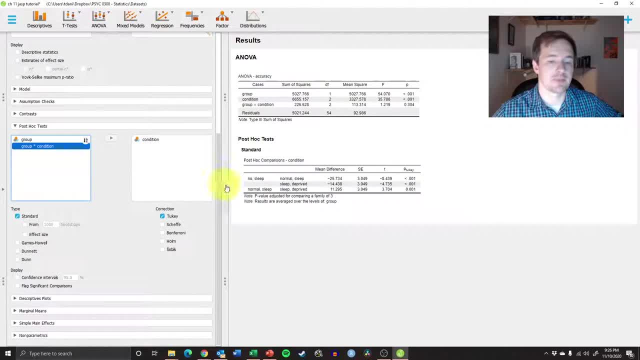 The way that we can find that out is to go to post-hoc drag over condition, and now you have this nice new table that tells you where those differences come from, And so we're going to go ahead and do that, And so what I'm looking at here is basically differences across every kind of group. 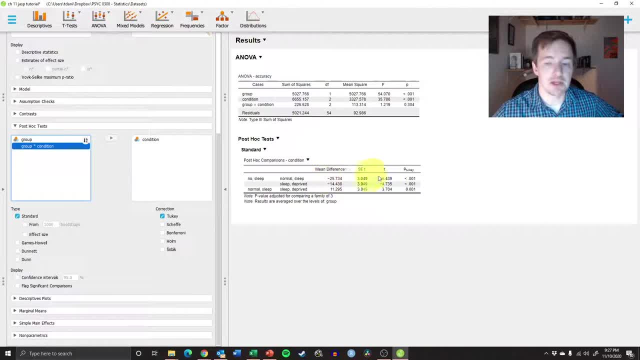 So if I'm comparing the no sleep with the normal sleep, you can see that it is significantly different. If I'm comparing no sleep versus the deprived condition, you can see that it is significantly different. The only one that's kind of close, I guess, to not being significant is the normal and the sleep-deprived conditions. 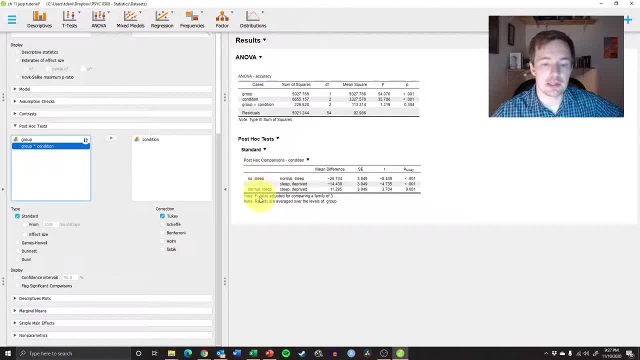 But you may be saying: but wait a second, What about the group? What about the groups? What about sober versus intoxicated? The way that you could look at that is moving that aside and then putting group by condition, because you want to look at both variables. 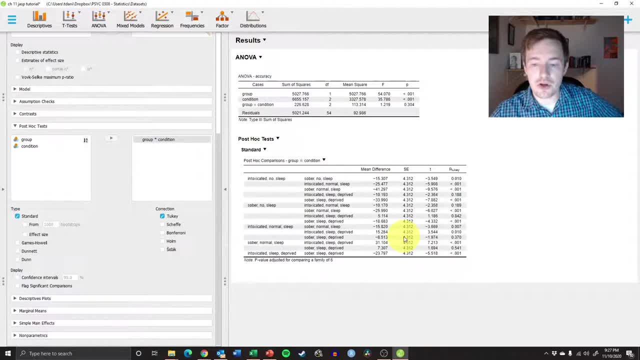 And then you can see all the different combinations here, And so we shouldn't really be looking at this just because we did not find this interaction variable to be significant. But just in case you want to explore the data a little bit, you can see that there are some. 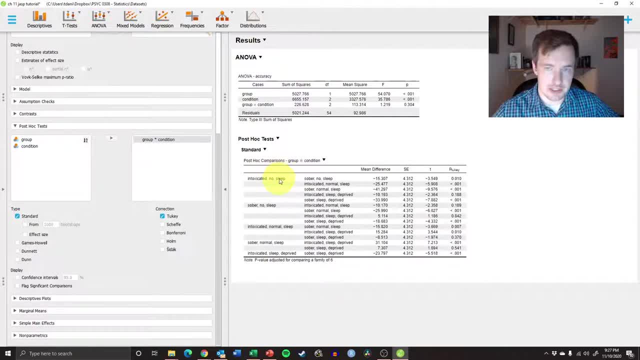 conditions that are not significant and some that are So. for example, I'm looking at intoxicated sleep. So the group is intoxicated, The condition is no sleep, And I can see that it looks like when compared to intoxicated sleep- deprived, there's not. 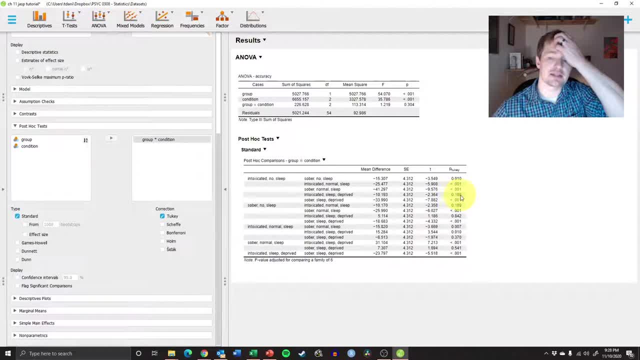 a significant difference. So that is you know. so that is interesting. But because this was not a significant factor in your ANOVA, you shouldn't really report this stuff without lots of qualifications. Here again we can see that sober and no sleep is not significantly different. 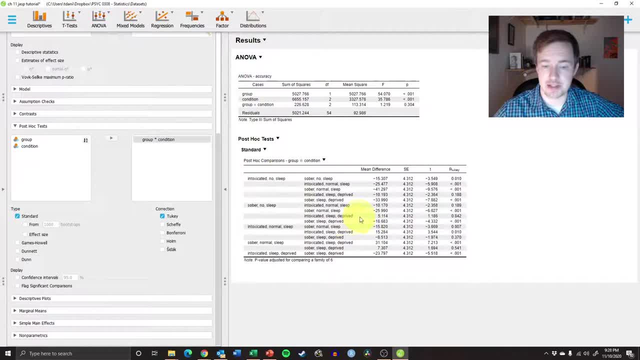 Okay, So this is different from sleep, this intoxicated, sleep deprived- And so you know, if I wanted to work a story up about this- which I shouldn't, because I just said that the rules are- you're not supposed to really dig into this too much, if you, if 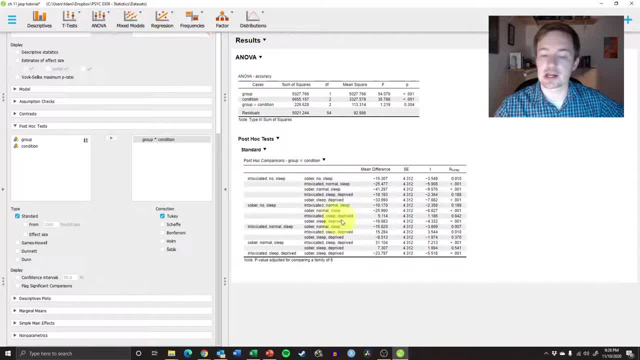 you don't have good reason to and I don't have good reason to. but I can see that intoxicated sleep deprived condition is not different from the sober no sleep condition, which must mean like, Ooh, maybe people do just as well when they're sleep deprived and intoxicated. 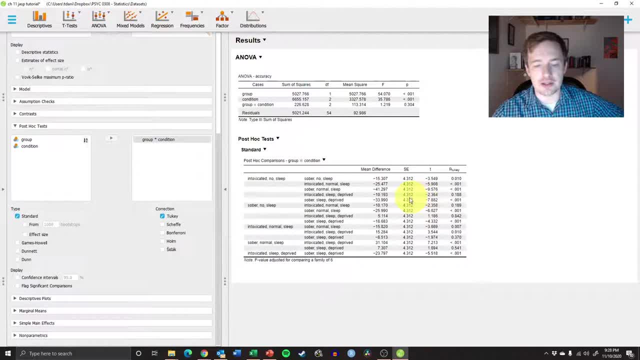 as somebody who is sober, who has not slept or something along those lines. Okay, But you can find lots of cool information here. One thing that I really love about JASP is its ability to toggle in and out of the the different postdoc connections corrections. 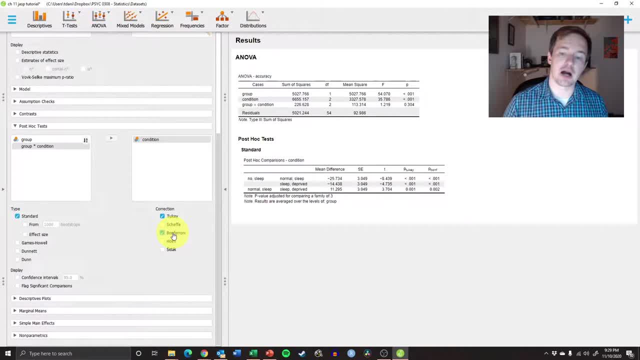 So usually two keys in bone Ferroni's are very popular postdocs and you can see how easy it is to compare those values whenever you are analyzing your, your postdocs here. If you'd like, you can also plot stuff in our. this one is a little bit harder. 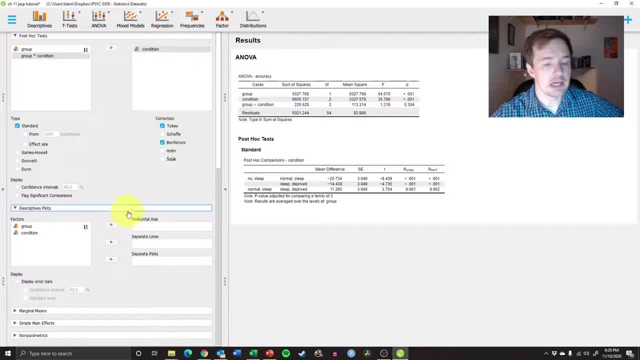 Okay, It's harder to interpret, so you might have to play around with it, but usually on the horizontal axis, you want what do you want your, what do you want your, your X axis to read as? So think about the factors that you want on your X axis. 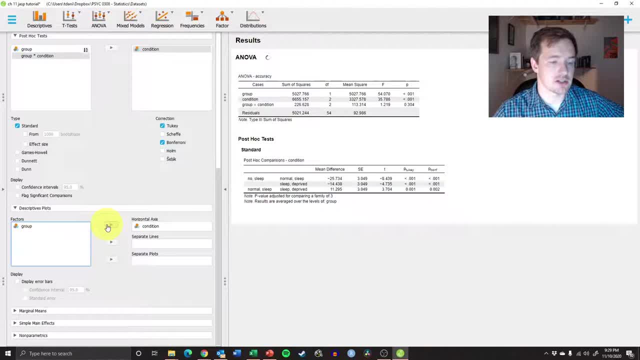 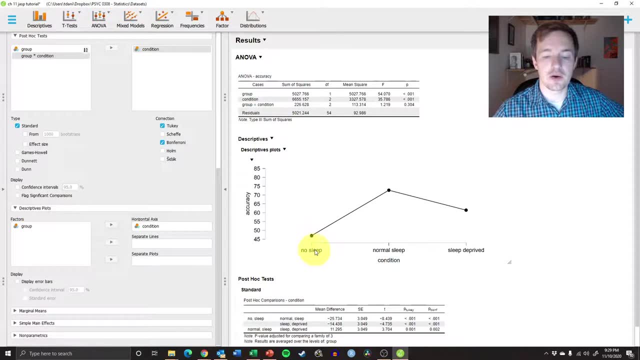 You can put that in the horizontal axis. I want my conditions here to be that, And so you can see right here plotting that data out. let's see there we go, That no sleep, normal sleep and sleep deprived. And if I wanted to, then I can also throw a group in as separate lines and you can see. 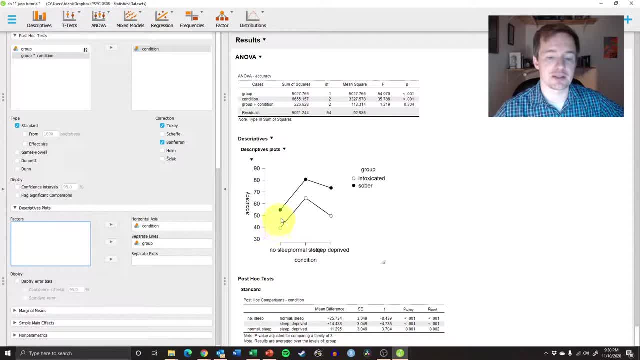 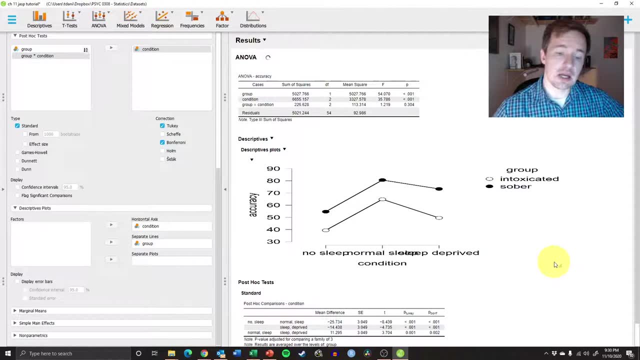 there. Yep, That does not look like an interaction, because these lines mostly look parallel. So we have the different groups right here, and so you can see how to read that as well. So you know the. the plots are not bad, you know, for they look much better than SPSS. 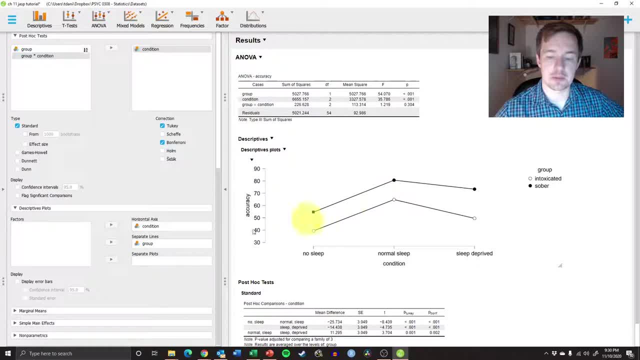 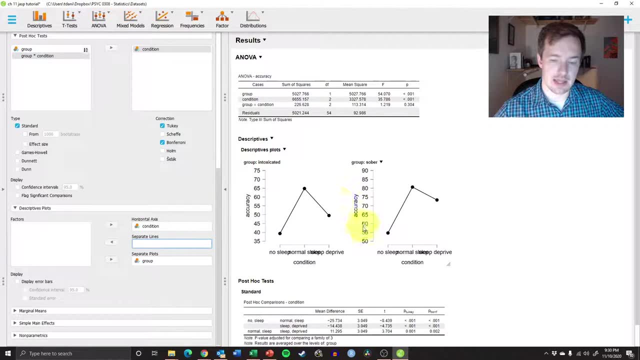 but if you did not want this data on the same, on the same scale, like this, you can always move it over to separate plots and that'll give you two separate ones. And there you go And you can see how the accuracy is very different there. 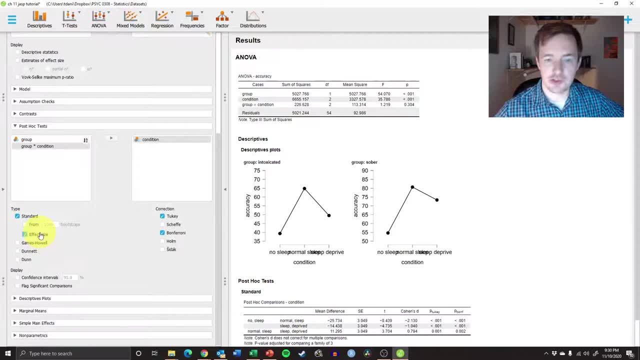 If you are interested in what else Effect sizes. you got your stuff here And and bootstrap there, But if anybody knows what these three things are, let me know, because I didn't learn that in grad school, So I can't tell you how to use those. 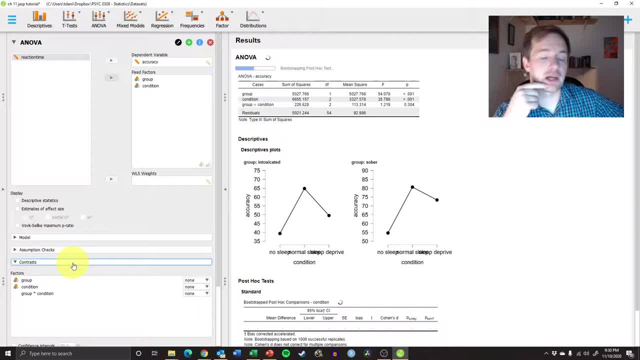 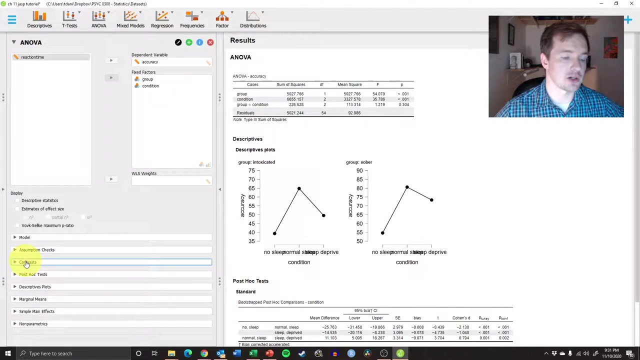 If you have specific ideas about the contrast here And basically what that means, Like if you had very specific predictions, a priori hypothesis predictions, then you could start moving around some of these weights to look at these separate contrasts- Not something you generally have to do unless your hypothesis calls for it. 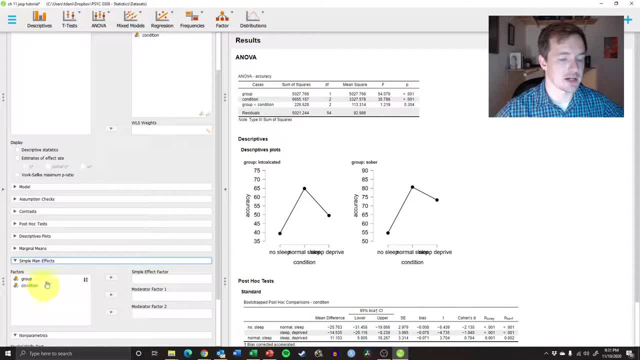 And we got some non-parametrics, some simple main effects, which are all helpful, but a little bit specialized, All right, so that's pretty much it. If you have any questions, let me know. Otherwise, thanks for tuning in. Bye.